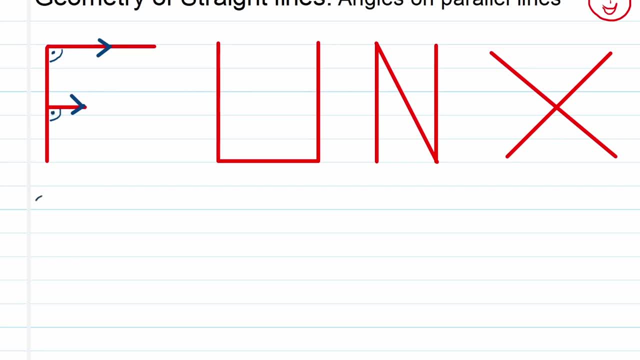 and that makes them equal. So the reason for that will say corresponding Corresponding angles. And very important. once you've used the reason for corresponding angles, it only applies to the purpose that you are considering those angles to be equal. Very important. Once you've used the reason for corresponding angles, it only applies to the purpose that you are considering those angles to be equal. 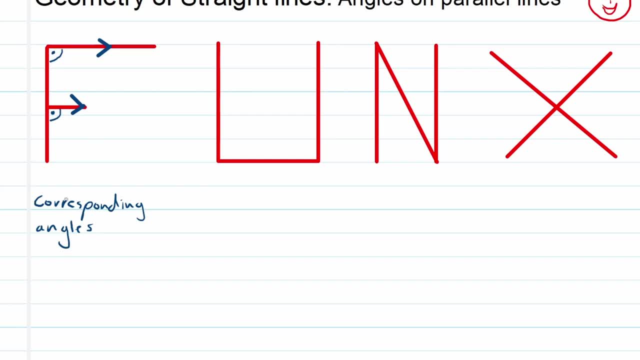 applies if there are parallel lines. so in your reasoning for geometry- anything that's called geometry- the moment you make a statement you have to give a reason. so you can't just make a statement. you have to make a statement and then give a reason. and once you give a reason here for corresponding angles. 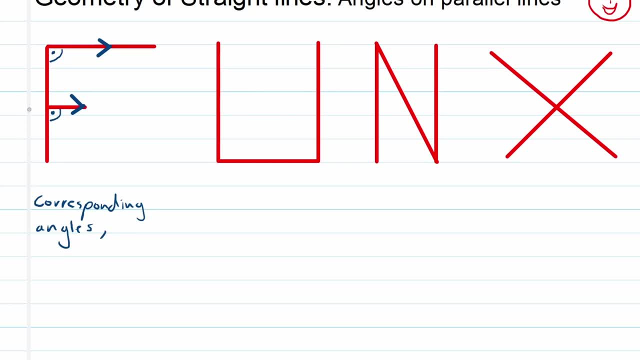 you have to say corresponding angles and then say which lines were parallel. so let's say it's A, B, C, D. so in this case you have to then say AB is parallel to C? D and that's important and that will help you to get full marks. second one: 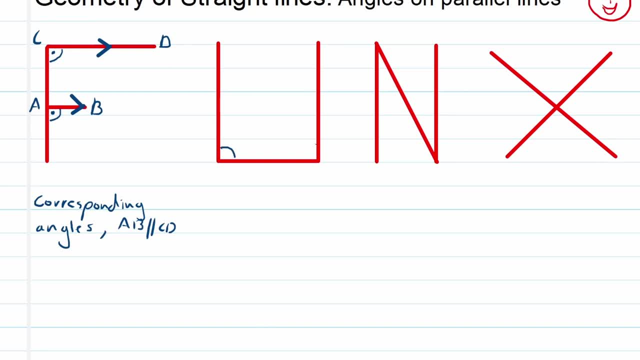 co-interior angles. this angle and that one are co-interior, and if they are co-interior they're not equal, but they are supplementary. what the word supplementary means is: they add up to all these points and if you want to be more specific, you can just say the. 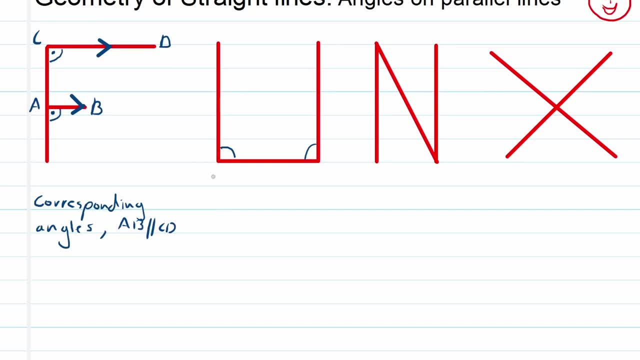 remaining three points are the same one and you might be wrong if they are similar to the previous different angle. you just say the remaining three points are 180 degrees. So let's say this is angle A and that's angle B. Let's say this is C and that's D. 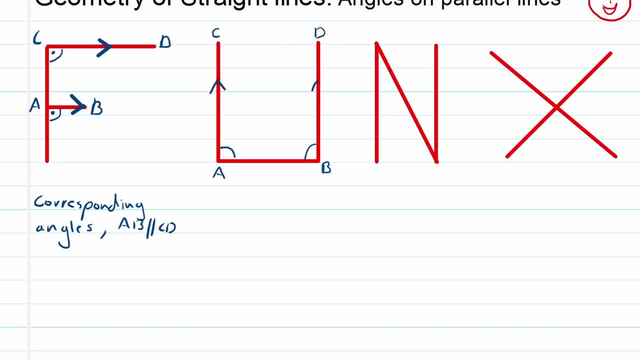 and remember: for this to be true, there have to be parallel lines. So AC and BD are parallel. Okay, so let's call this angle A and we call this B1, and just for the sake of explanation, I'm going to draw a little line there and call this B2.. Now, from here, the very first one, you 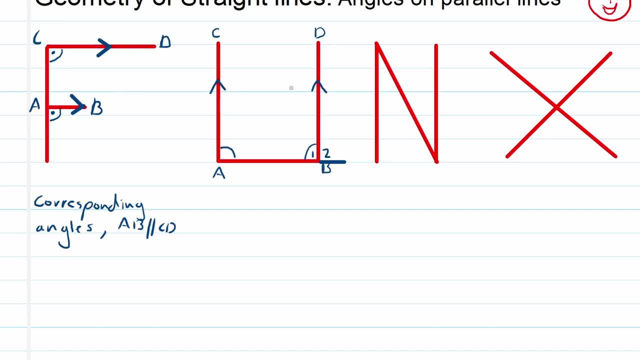 know these are corresponding. So in this example at the U for fun, A and B2 are equal as well. right, But we know B1 and B2 are angles in a straight line, which makes them add up to 180.. So if B2 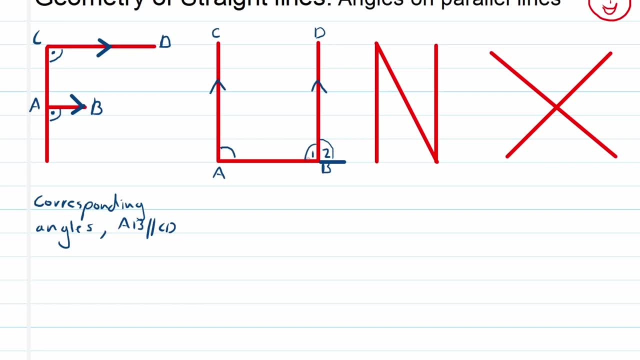 is equal to A and B1, and B2 adds up to 180. that means that B1 and B2 are angles in a straight line and A also add up to 180. So we say co-interior angles, Co-interior angles. 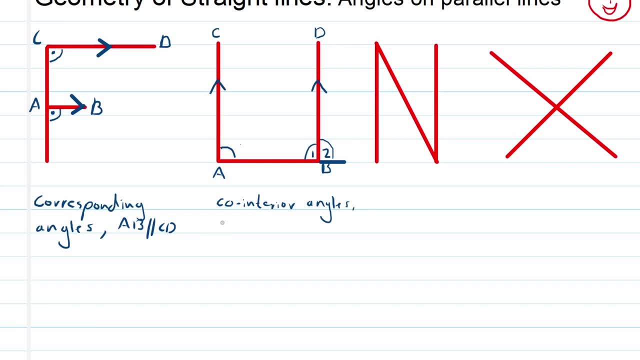 Remember, when we use this, we have to state which lines are parallel. That's very important. So that's your full reason. Any statement needs a reason and the moment you use parallel lines, you have to state the half parallel. So that's the U. for fun, Let's go to the end. part of fun. These two angles are something we 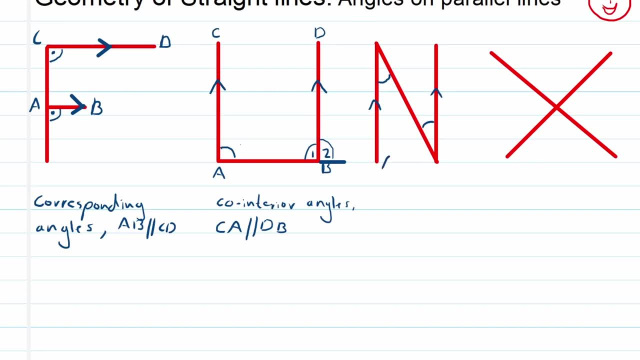 call alternating angles. Let's again call this an: A, B, C and D. Angle B and angle C are equal. Why? Because they're alternating angles. Just to complete the reason, here I would say: angle A is equal to angle C. Over here we will say: angle A plus B1.. Adds up to: 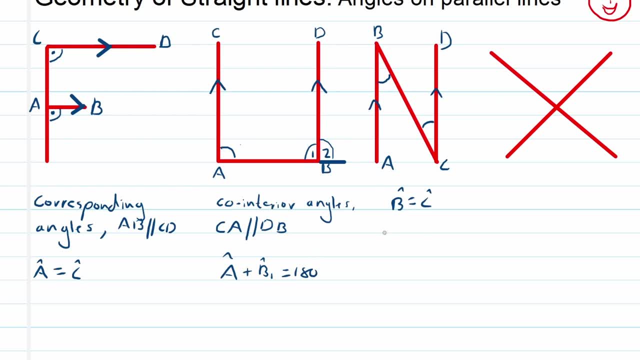 180.. Over here, B and C are equal, So we will say alternating angles. Remember this only applies if there are parallel lines. So we have to say here that A, B is parallel to C, D, Very important. So we've done the fun part in math. Let's 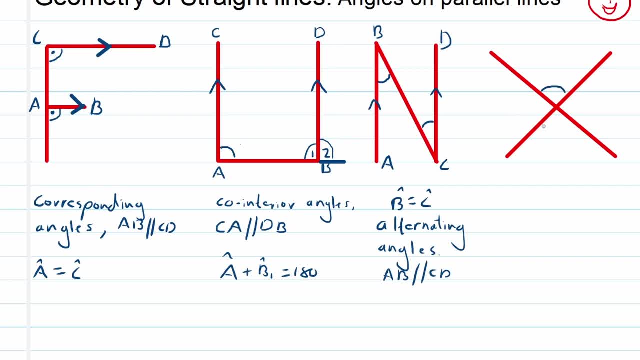 go to the X factor, And that's the one we've already mentioned Vertically opposite. Okay, This has nothing to do with parallel lines, So I'm just going to separate it right there, But keep in mind this is a way for you to remember it. So fun, Maths is fun, and it has. 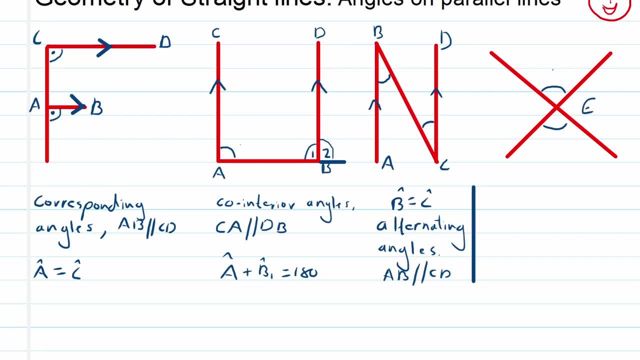 an X factor to it. So let's say this is E1, 2,, 3 and 4.. As stated already, E1 is equal to E3. And we know E2 is equal to E4. The reason over here is vertically opposite.